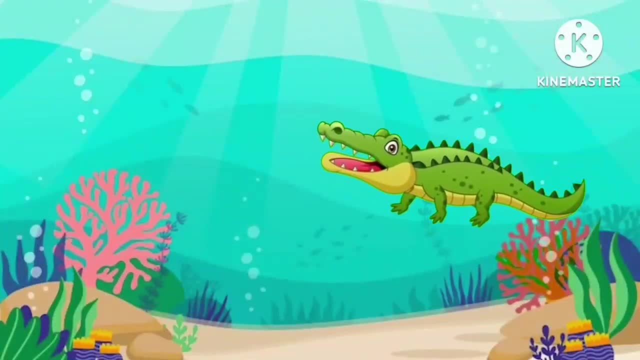 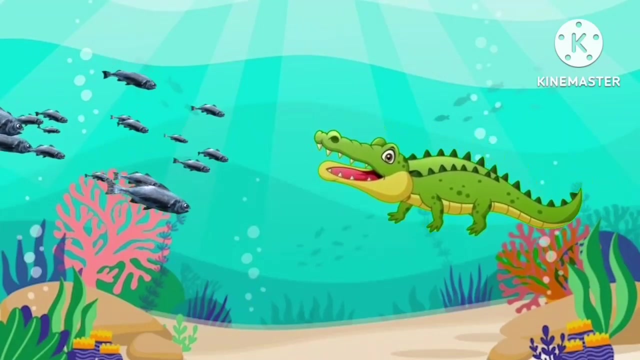 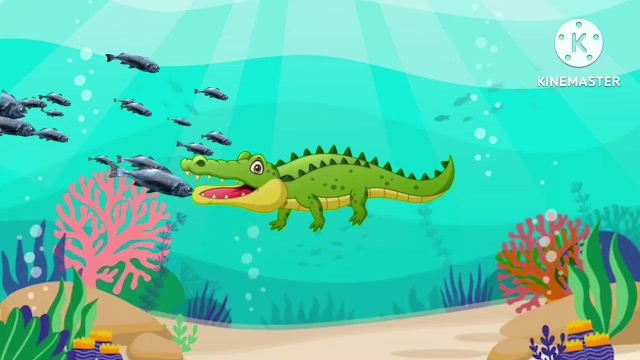 Yay. One day Mr Crocs is hungry for lunch, He wants to eat fish. So he is looking for the biggest number of fishes to eat. For eating more fishes, he is opening his mouth Finally. he finds more fishes And eat them up. 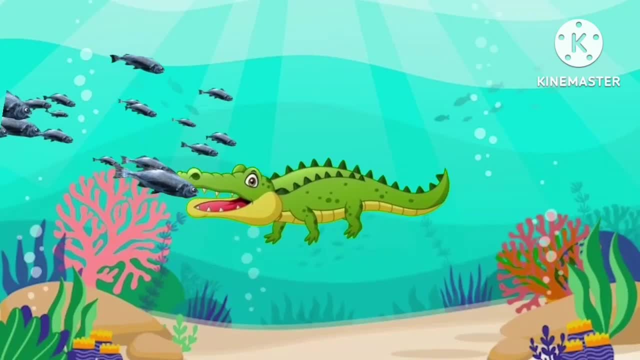 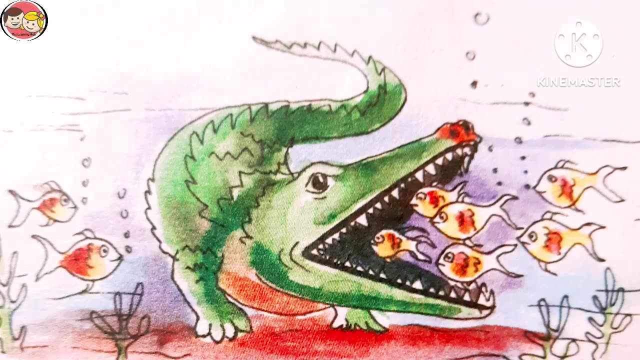 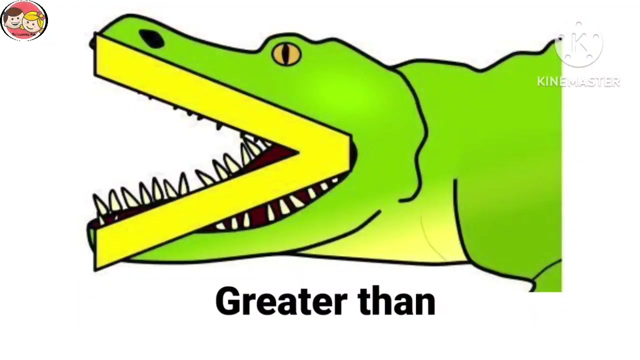 Munch, Munch, Yummy, And at last he gets very happy. So, children, the hungry Crocodile always likes to eat a large number of fishes. So the open mouth of the Crocodile indicates the symbol greater than or less than. this sign represents greater than and. 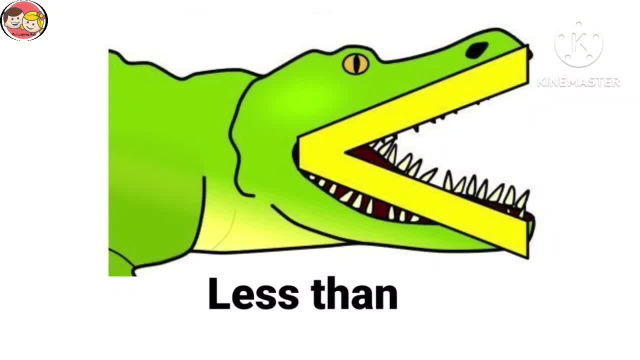 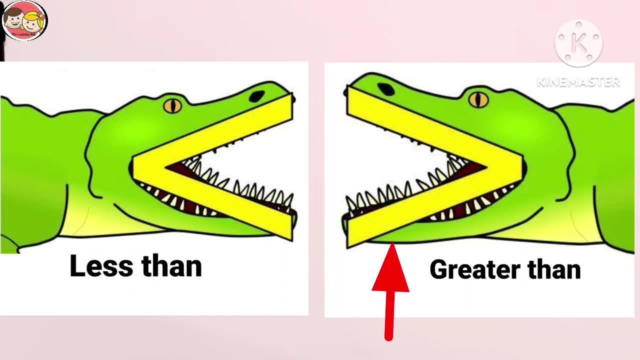 this sign represents less than children. look here and observe very carefully. this is greater than sign and this is less than sign children. we need to remember that, as mr Crocs always wants to eat a large number of fishes, so the crocodile's mouth always opens towards the biggest number. now, how do you? 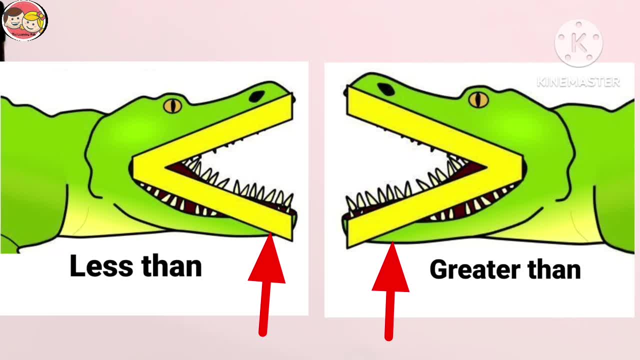 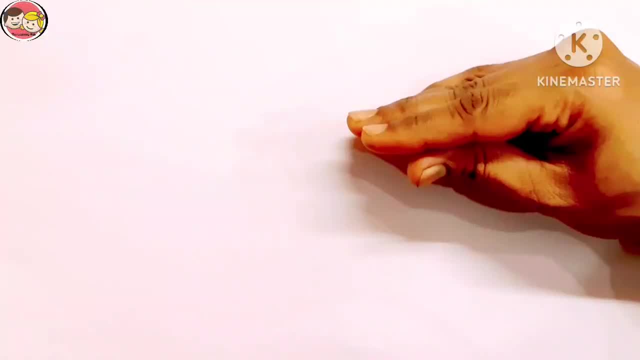 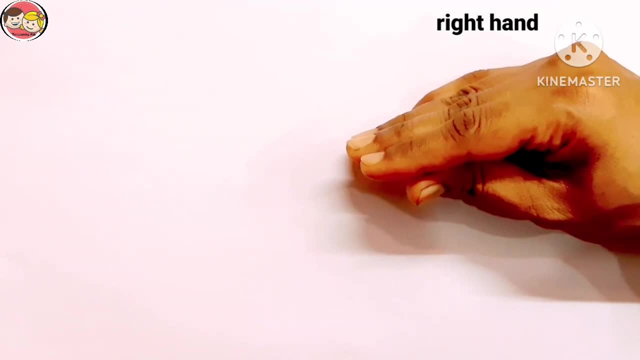 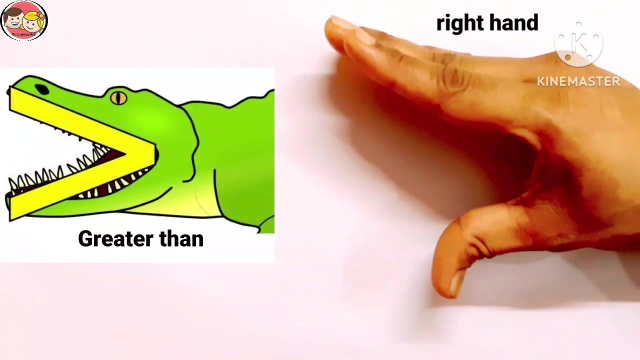 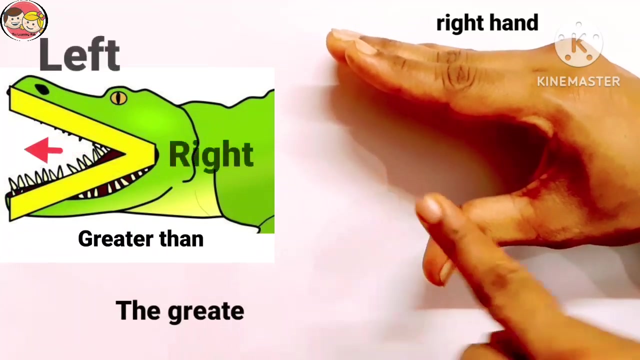 remember which one is greater than and which one is less than sign. for that we need to use our hands. children, look here and observe very carefully you. if we make an open crocodile mouth with the help of right hand, it becomes greater than sign. look here, this is greater than sign. the mouth is open in. 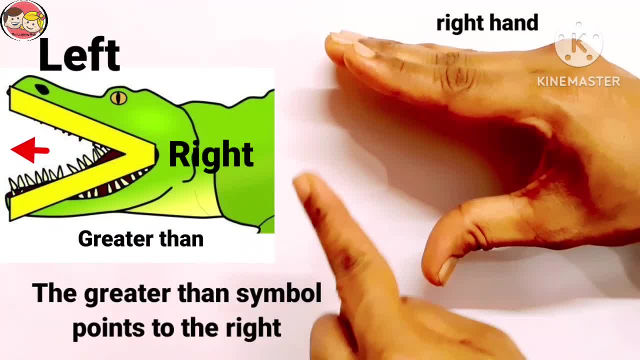 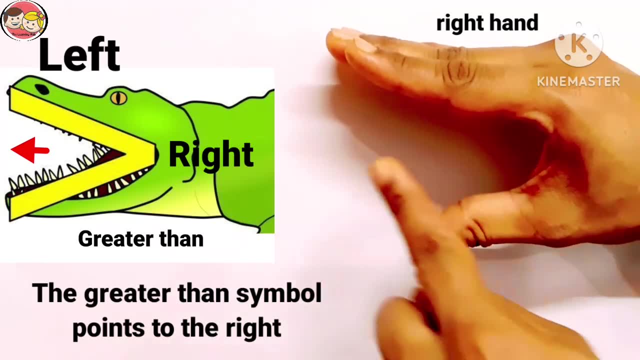 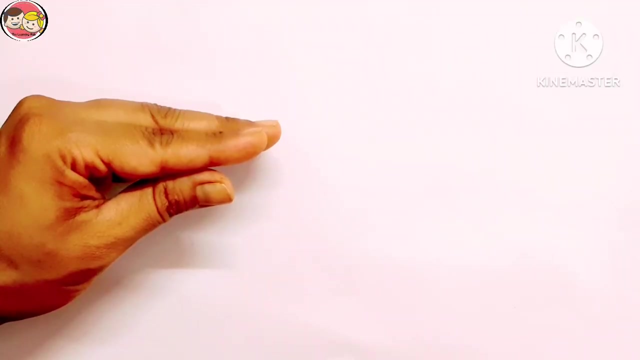 this direction. that means the bigger number is here only and there is smaller number in this side. open mouth always indicates, indicates the bigger number, so this is greater than sign. this is greater than sign now if we make an open crocodile mouth with the help of left hand, like 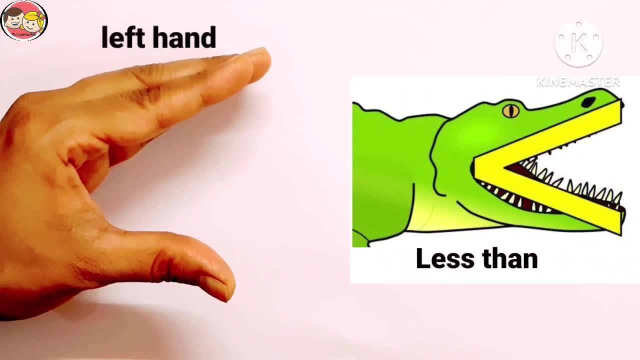 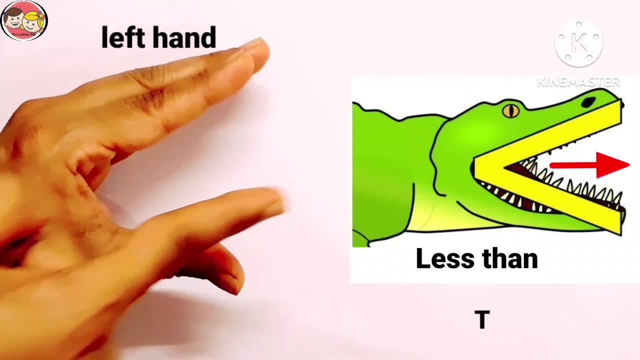 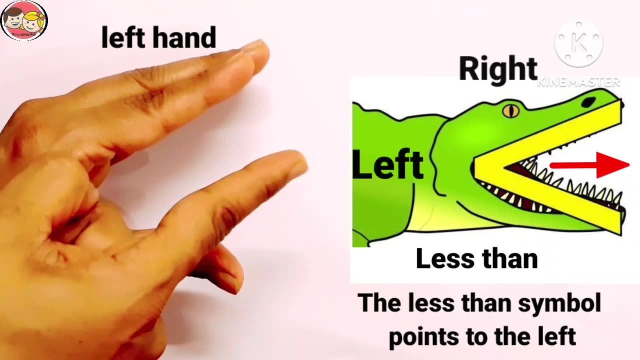 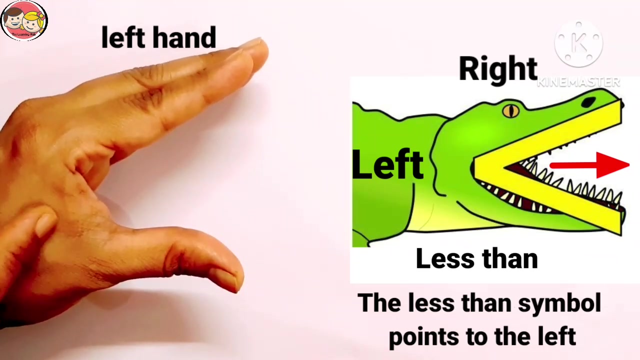 this, it becomes less than sign. look here, this is less than sign. the mouth is open in this direction. that means the bigger number is here only. open mouth indicates towards the bigger number and the back of the mouth points towards the smaller number. so there is smaller number in this side. so this is less than sign with sign, less than sign. so, children, we must. 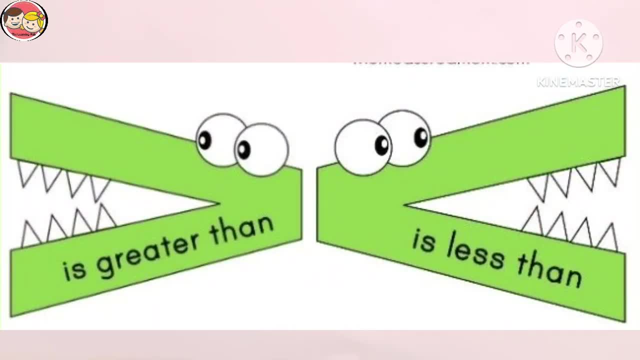 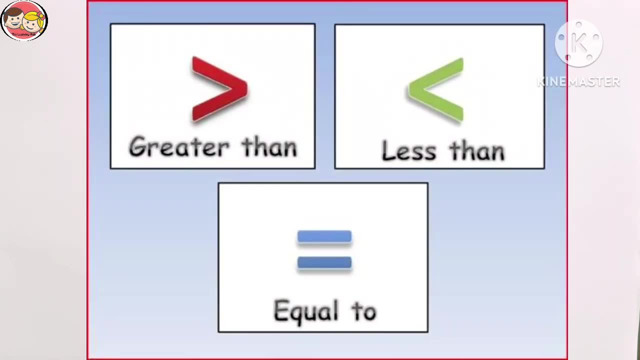 always remember that the crocodile's mouth always opens towards the bigger number. so greater than, less than and equal to symbols are used to compare any two numbers. when a number is bigger than or smaller than another number, then greater than or less than symbols are used if the first number 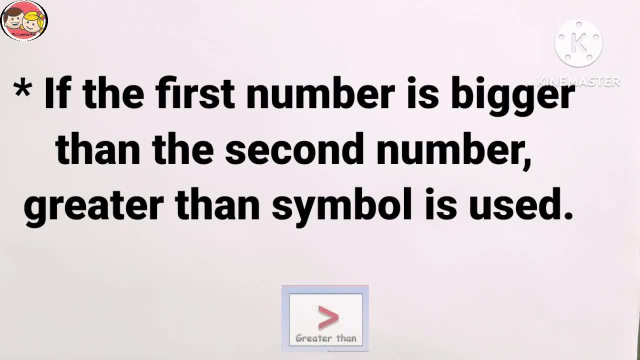 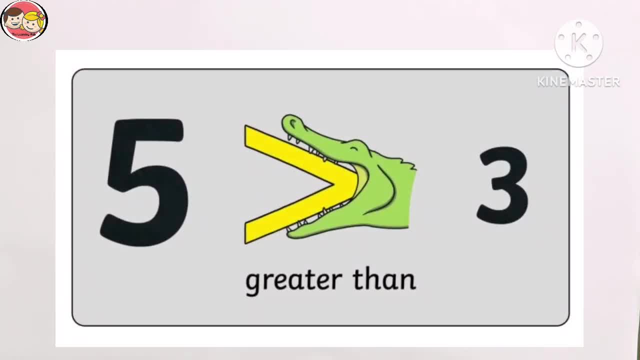 is greater than or less than, then greater than or less than is used to compare any two numbers than the second number. then greater than symbol is used, for example five and three. there are two numbers, five and three. now tell me which one is greater number? yes, the first number, five, is. 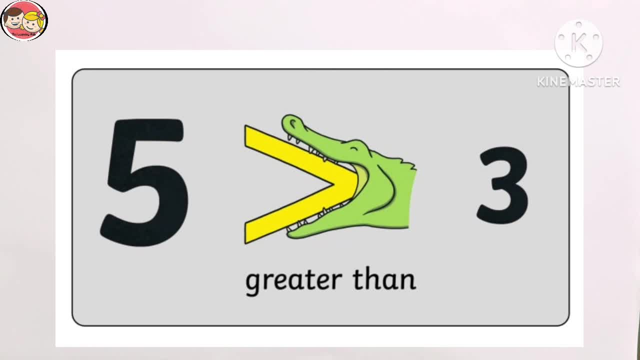 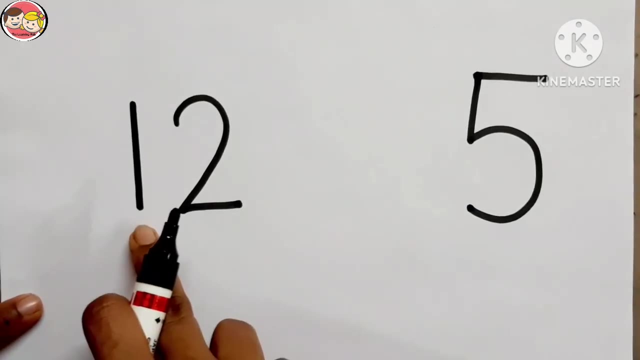 greater number. so number five is greater than number three. so here we need to put the greater than sign. greater than number three, we can also put the greater than symbol, so here we need to put children. one more example: look here there are two numbers. first number is 1 to 12 and the second one. 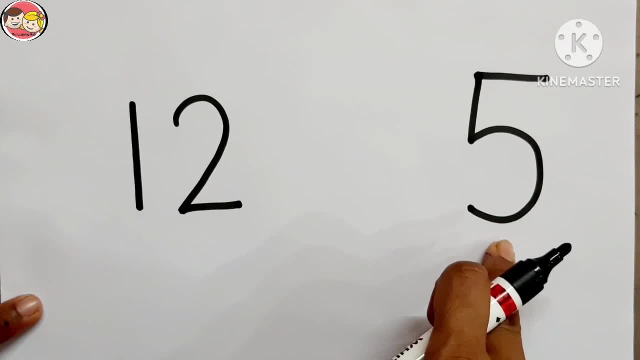 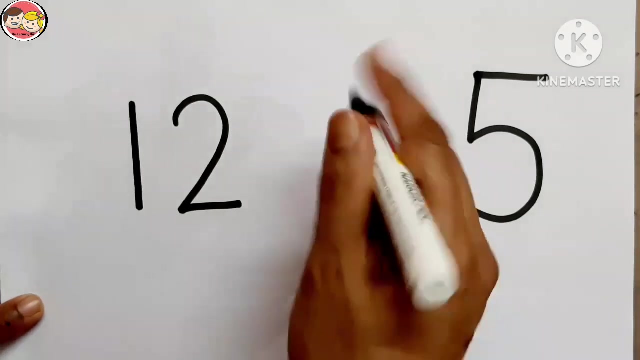 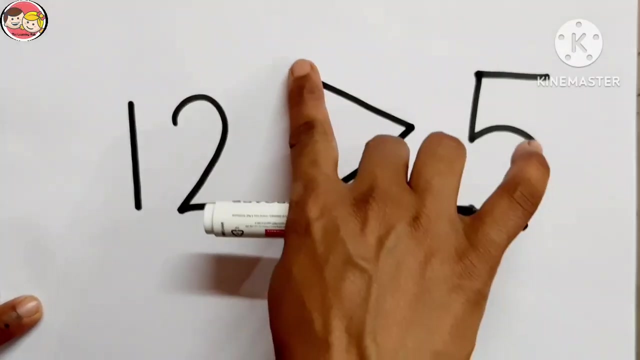 is number 5. now tell me which one is greater number. yes, number 12. the first number, 12, is greater number. so 12 is greater than number 5. so here we need to apply fish sign. very good, greater than sign. this is greater than sign. the hungry crocodile is opening his mouth towards the 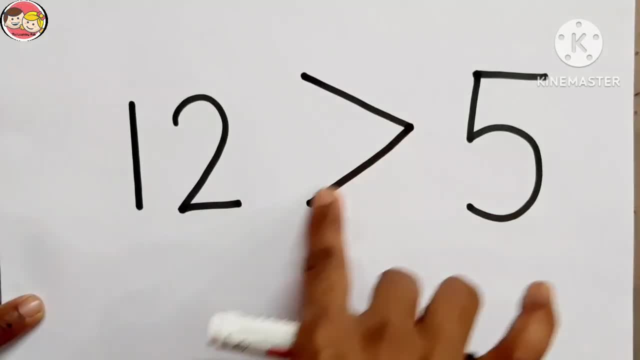 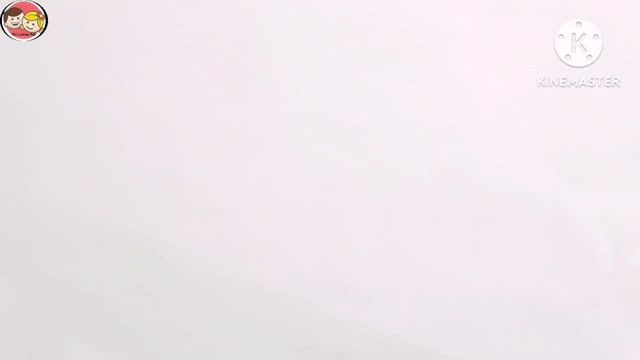 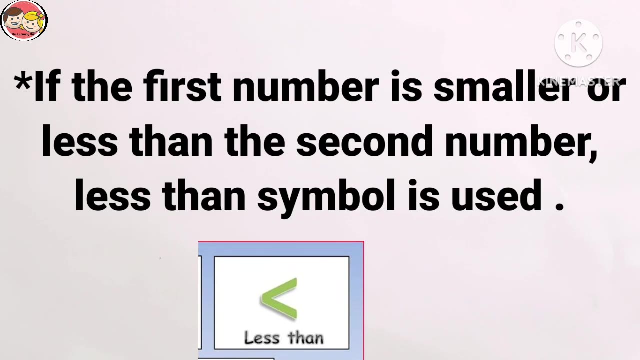 bigger number. so this is greater than sign. number 12 is greater than number five. Next, if the first number is smaller or less than the second number, then less than symbol is used. I repeat: if the first number is smaller or less than the second number, then less than. 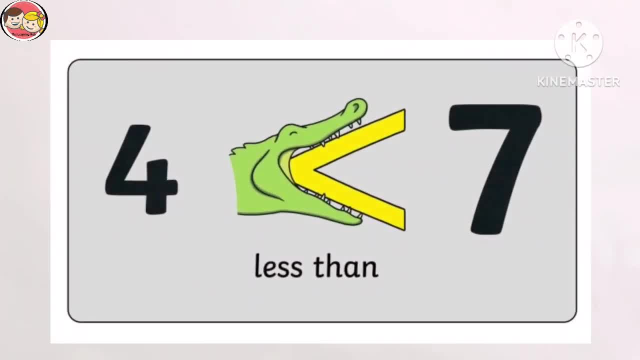 symbol is used. Look here: number four and seven. There are two numbers, four and seven, Here the first number is 4 and the second number is 7. now tell me, which one is smaller number. yes, number 4 is smaller number. it means number 4 is less than number 7. so here we have to put less than sign. 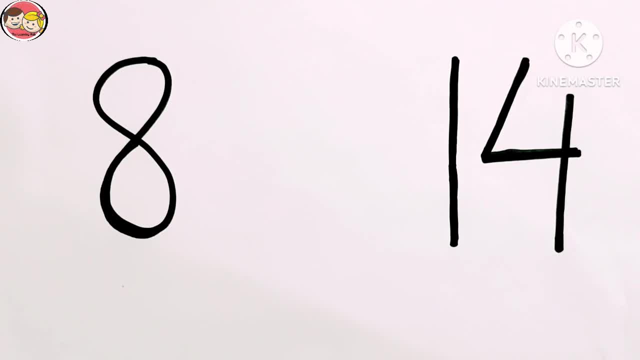 now look at the next example. there are two numbers, number 8 and number 14. 1, 4, 14. now tell me which one is smaller number. yes, number 8 is a smaller number. the first number is 8 and 8 is smaller number. so the number 8 is less than number 14. so here we have to put less than sign. this is: 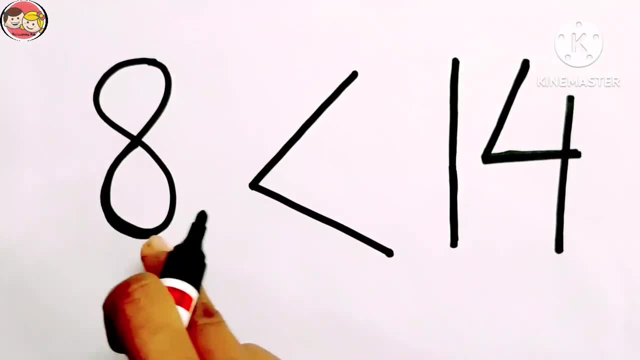 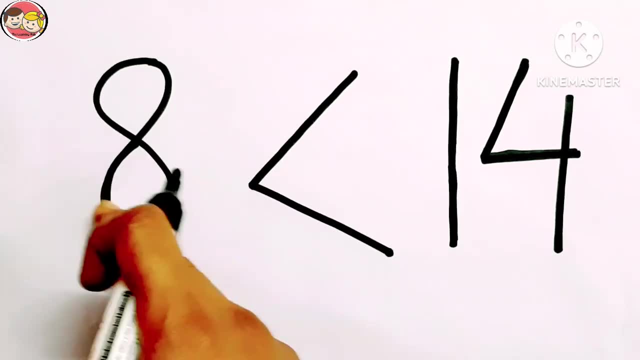 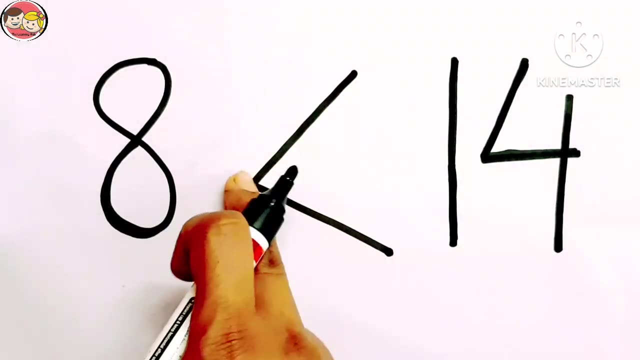 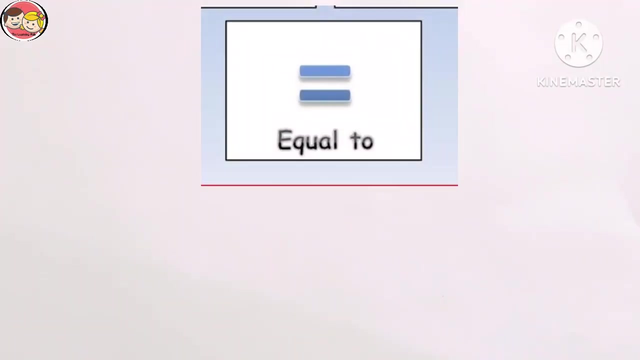 less than sign. so number 8 is less than number 14. less than symbol always points to the smaller value. Less than symbol always points to the smaller value. So this is less than sign. Number 8 is less than number 14.. Next, this sign represents equal to. The equal to is used to show. 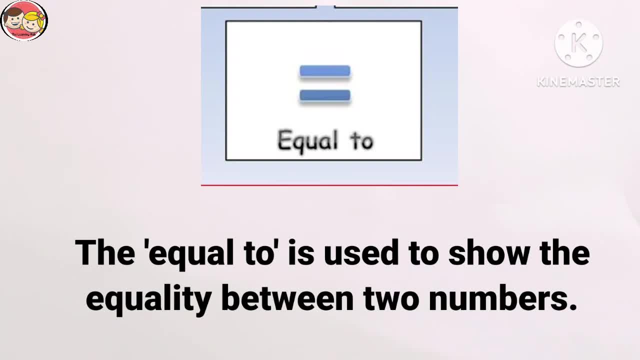 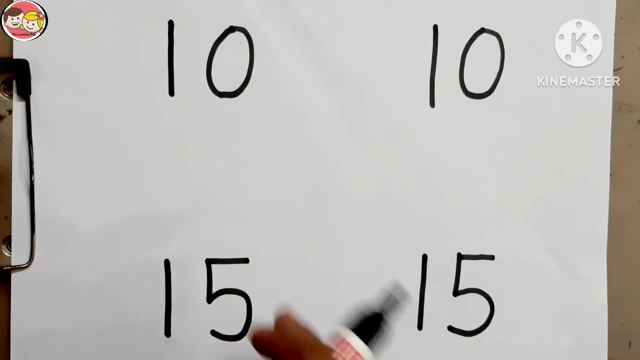 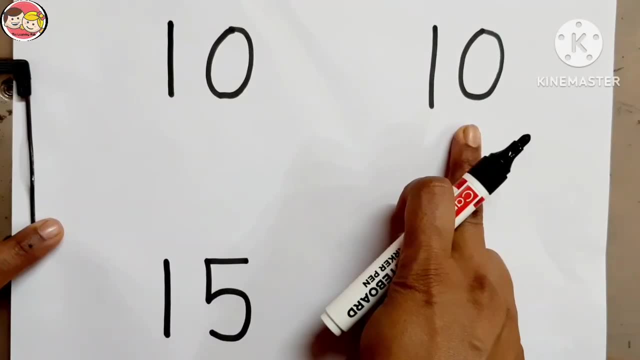 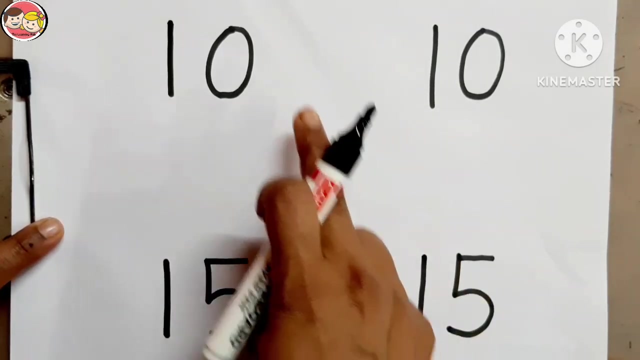 the equality between two numbers. It means that the numbers on the both sides are the same. Children, look here. There are two numbers. The first number is 1010 and the second number is also 1010. So here we can easily see that both numbers are same means equal. So here we need to apply. 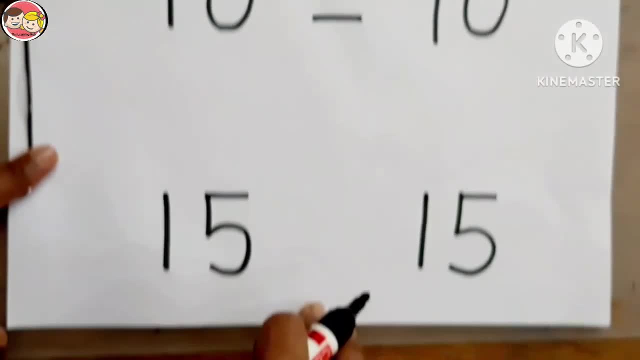 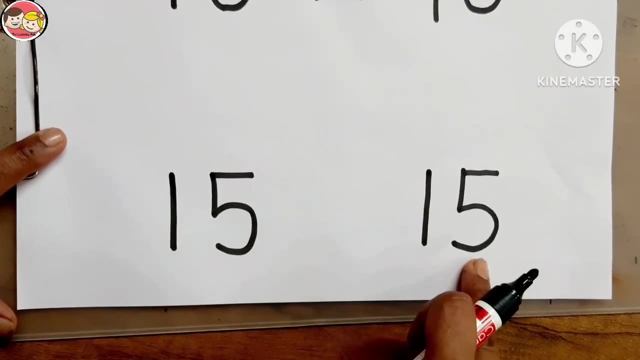 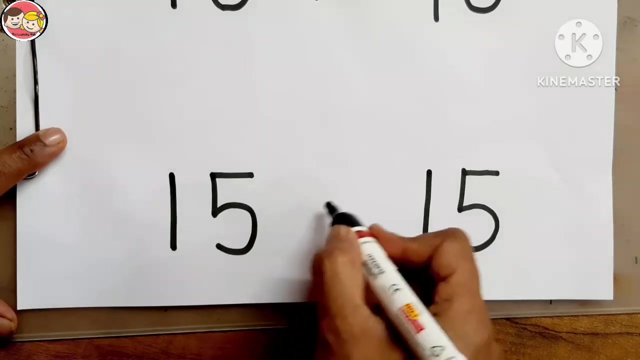 equal to sign. Now look at the next example. The first number is 1515 and the next number is also 1515. So both numbers are same, means equal. So here we need to apply V sign: Yes, equal to sign. Now let 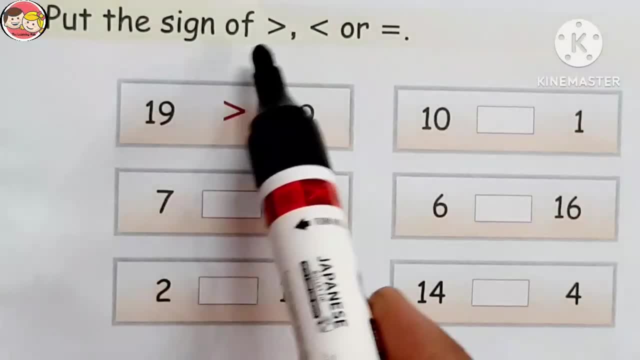 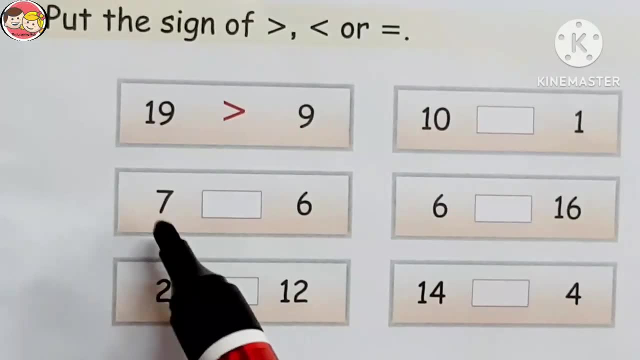 me check how much you have learned. Put the sign of greater than, less than or equal to number 7 and 6.. Look at the first number, number 7.. Number 7 is bigger than number 6.. So here we need to apply. 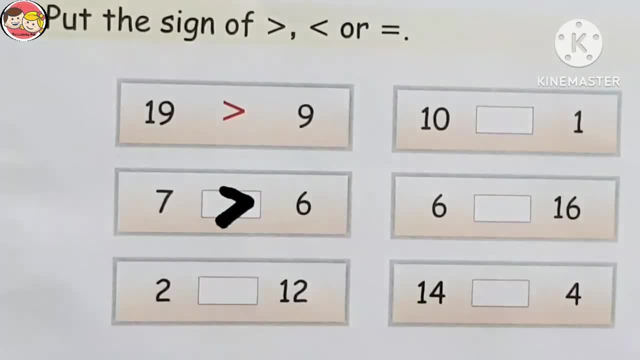 greater than sign. If the first number is greater than the second number, then we have to put the greater than sign. Now look at the next example. The first number is 2 and the next number is 12. So 2 is smaller than number 12.. 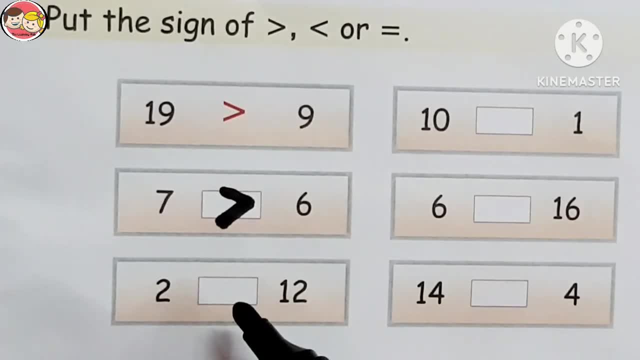 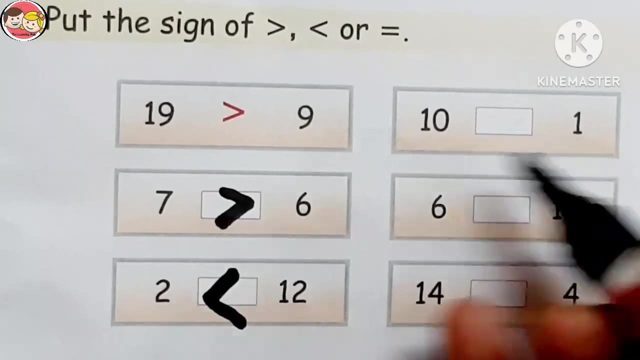 Means here we need to put V sign. Very good, Less than sign. Number 2 is less than number 12.. Now look at the next example. number is number 10 and the second number is 1, so first number is greater than number 1, so here: 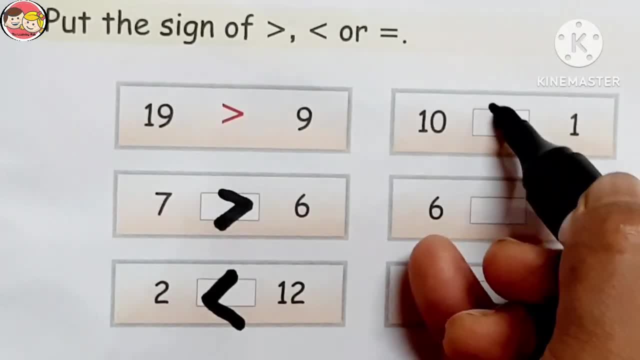 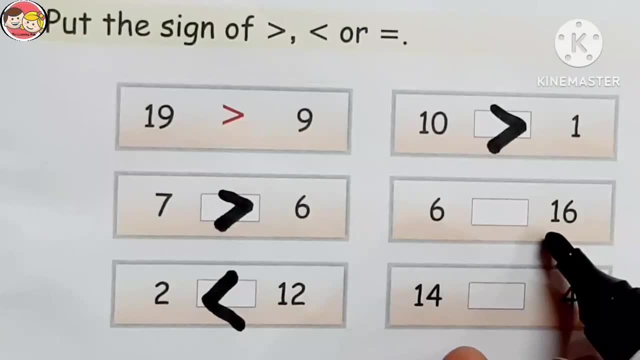 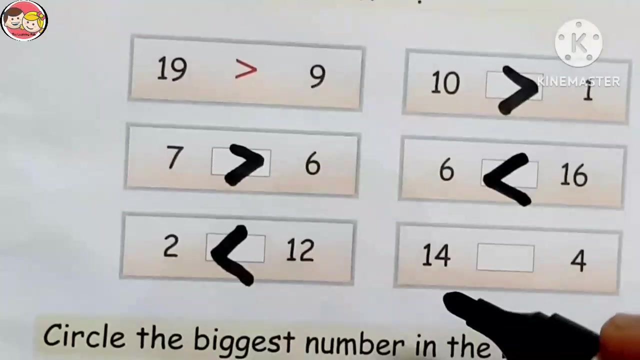 we need to apply with sign very good- greater than sign. now look at the next example. the first number is 6 and the second number is 16. so first number 6 is smaller or less than number 16. so here we need to apply less than sign. now look at the next example. first number is 1 for 14. 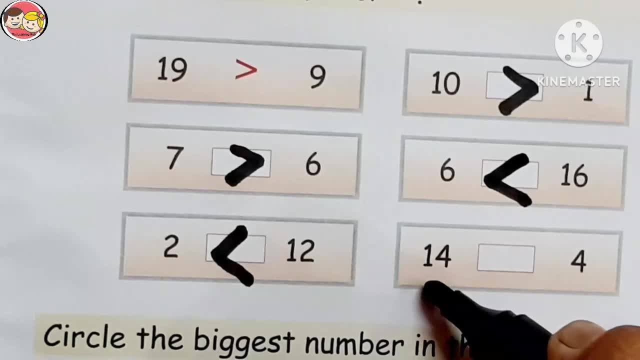 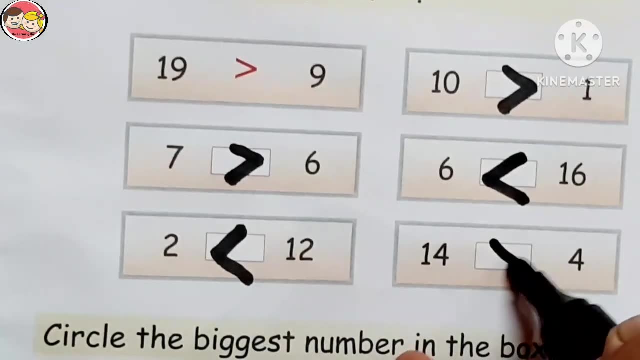 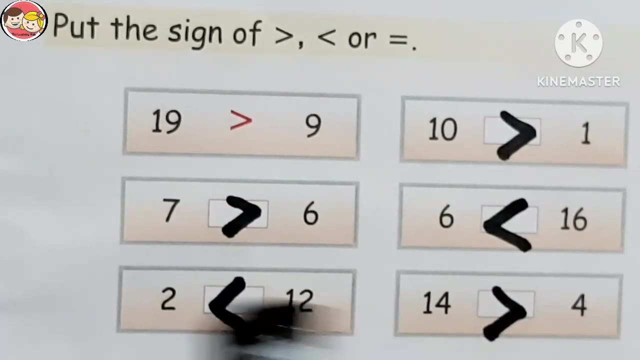 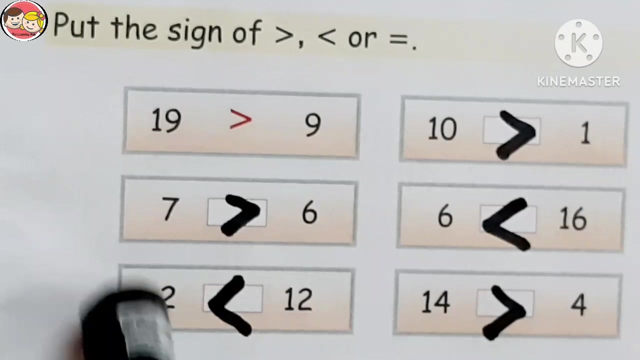 and the second number is 14 is greater than number 4. so here we need to apply greater than sign doing. it's a very important topic, but don't be confused. you only need to see at the. you only need to see at the first number. if the first number is greater than the second number, then you have to put greater.